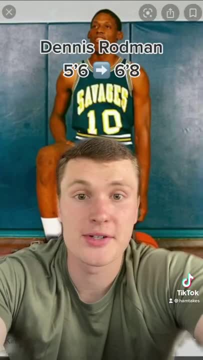 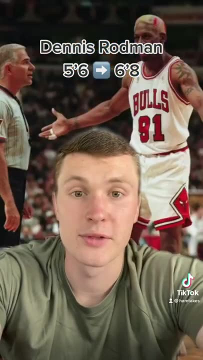 Hopefully the same happens for his son. Dennis Rodman got cut from his varsity team and graduated high school at 5'6.. When he was 19, he had a growth spurt to 6'8.. This man grew 14 inches in. 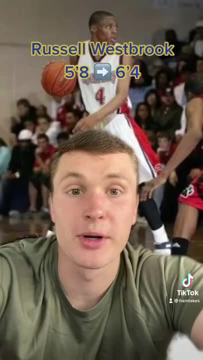 one year. That might be the strangest thing about him, Russell Westbrook. his sophomore year, high school, was only 5'8. And at 5'8, he could windmill. Now he's 6'4 and a nightly triple-double. 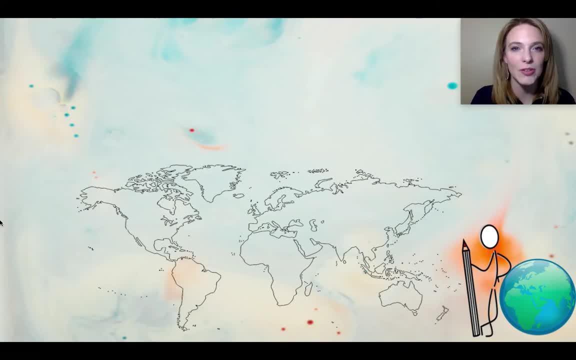 Hi guys, welcome back to geography class. We're going to pray in and get started. Dear Heavenly Father, Lord, I just pray that you will be with us throughout this class period, that you'll be with my students as they're watching this video. I pray for a hedge of. 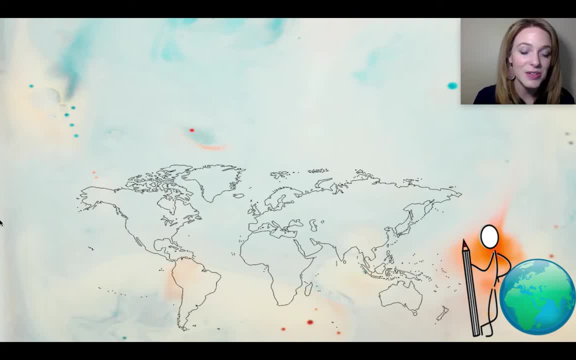 protection around them. Lord, as this is a unique time in life where we just ask for your guidance, your wisdom, your discernment. Lord, I pray that you'll keep our hearts soft so they can be molded by you. Keep us on the right path, Lord. Give us the desires of our heart and let 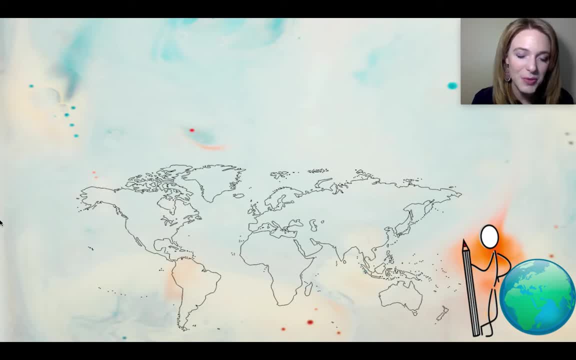 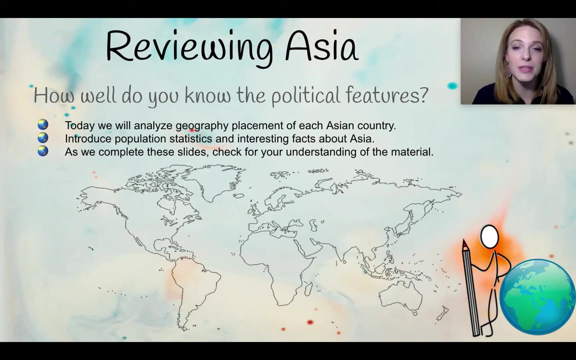 that be to glorify you, Lord. We love you so much. In your son's name we pray Amen. Today, we are going to be reviewing the political features within Asia. I'm going to introduce the geographic placements, as well as some interesting statistics and facts. 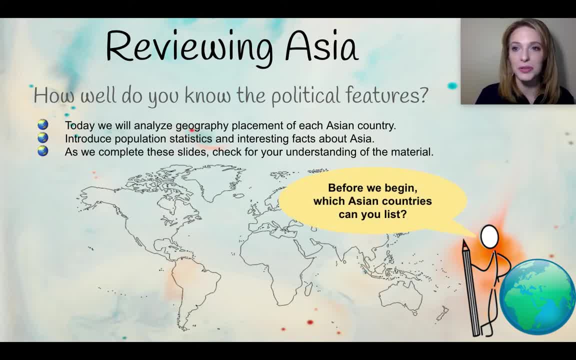 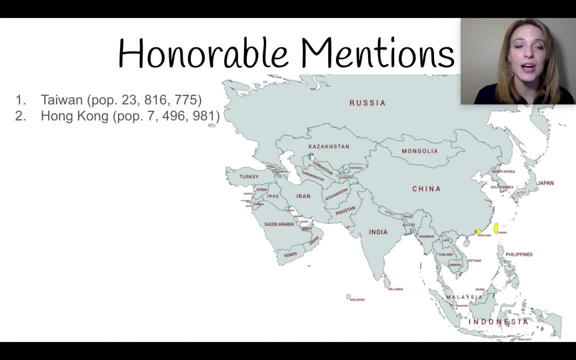 Before we begin, which Asian countries can you list? Honorable mentions: Taiwan and Hong Kong do have a significantly high population, and yet they're not countries. They are considered to be something we call dependencies, and specifically dependencies of China. Now let's move on to the countries. 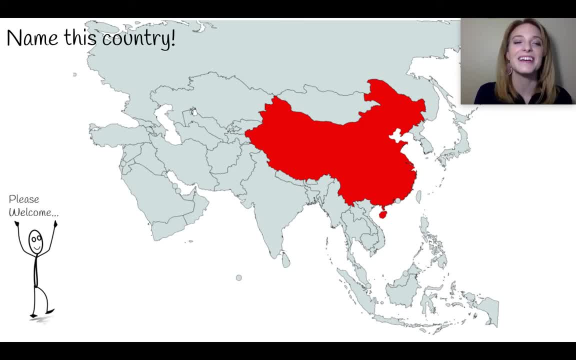 Can you name this country? I bet you can. So please welcome that guy. He's going to be the one giving us interesting facts and example. In this country we have a population that is over one billion. And then also, please welcome answering Karen. She's going to be the one giving you the answers to the countries. Of course, this is China, most definitely, And if you were to do the math today, in 2020, we would have following leaders: your country that we think would be the most likely. What would you think? There's a lot of jobs to be found. Of course. that should list out like as many as fuckin'.